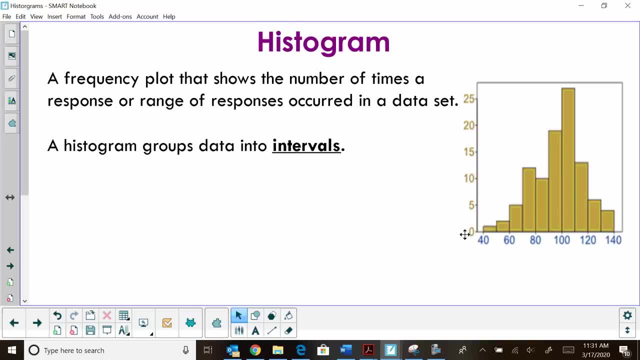 On the y-axis I have intervals marked in fives: 5, 10,, 15,, 20, 25.. So when I go to interpret this, I'm going to have to think of an interval. So what? how many responses were between 50,- I'm sorry, 60 and 70, and the answer would be 5.. 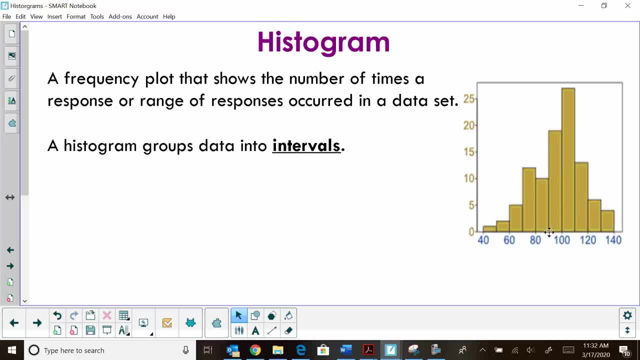 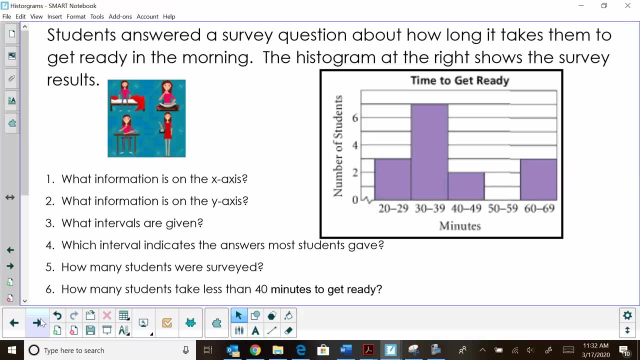 How many responses were between 80 and 90, and that answer would be 10 responses. So we're going to interpret this. Here is our first question. Students answered a survey question about how long it takes them to get ready in the morning. 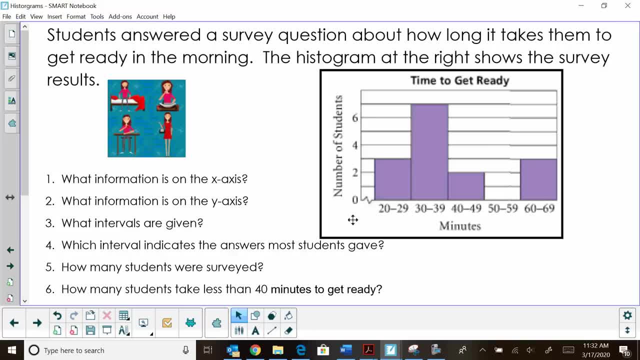 The histogram at the right shows the survey results. So let's look at the questions. use our histogram to answer those. What information is on the x-axis? So let's look at the question. So let's look along this X axis. Well, what information are the minutes? 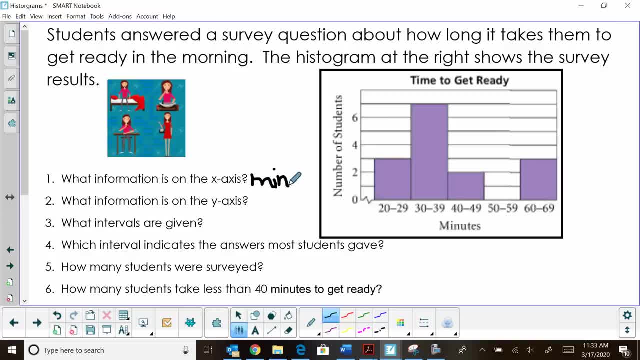 that it takes a student to get ready. So the minutes to get ready. Okay, what information is along the Y axis? Well, this is how many students responded, or the number of students. So I'm just going to put, for space sake. 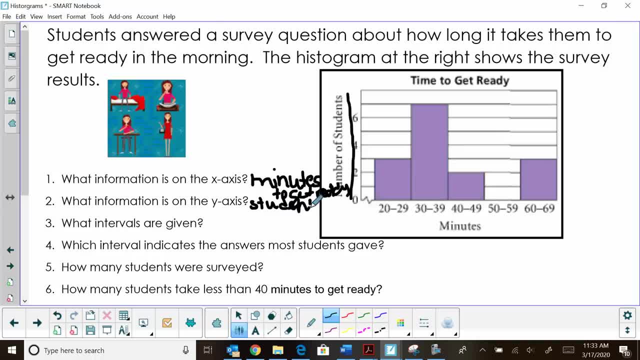 just the word student responses, or the number of students. Okay, so our X axis represents the time and the Y axis represents the number of students that responded to those times. Question three: what intervals are given? Okay, so, on a, On a histogram you're not going to have. well, it took me 21 minutes to get ready. 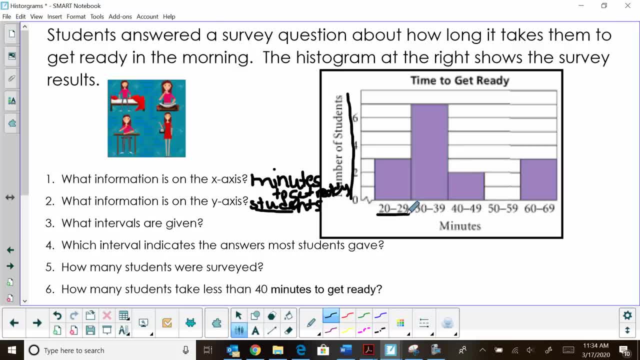 It's an interval and in this case from 20 to 29 minutes. So they're in 10-minute intervals, 30 to 40 minutes, 40 to 50 minutes, 50 to 60 minutes and 60 to 69 or 70 minutes. 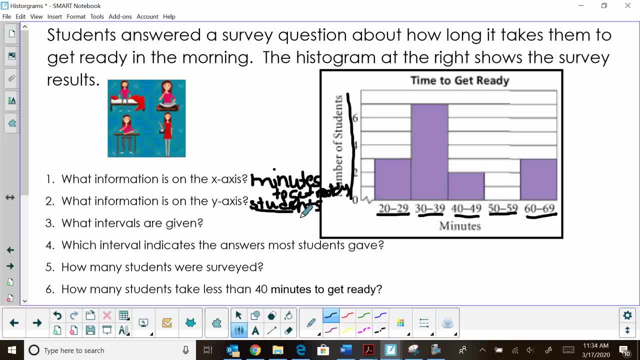 So you've got these intervals of 10 minutes. So what are the intervals? They are in 10.. That's right. 30 to 40 minutes intervals. Okay, which intervals indicate the answer most students gave? Okay, so we're looking for what's called the mode which answer occurred the most? 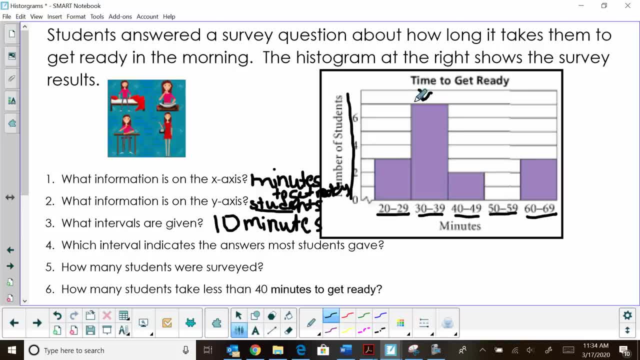 Well, that's easy, because it is always the tallest bar in our histogram graph. So the 30 to 39 minute interval is our most occurring answer. How many students were surveyed? Well, what you have to do for the total number to figure out how many students were surveyed is a look at how many students. 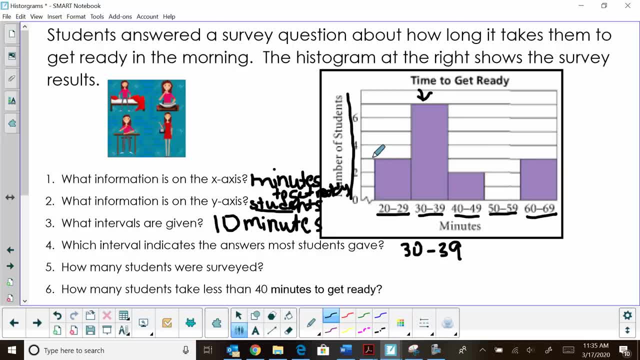 answered the question in each interval. So for the 20 to 29 interval we had three students that answered in that interval 30 to 39, we have how many, And that goes over here. Seven students were in that interval 40 to 49, we have two. Nobody answered in the 50 to 59. And then 60 to 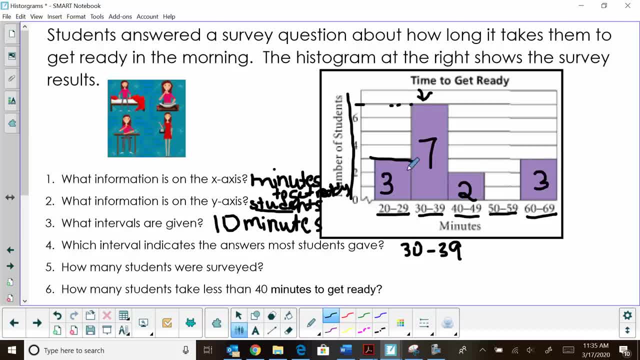 69, we had three students, So we're going to add all those up. Three plus seven, that's 10.. 10 plus seven, that's 10.. And we're going to add all those up And we're going to add all those up, And we're going to add all those up And we're going to add. 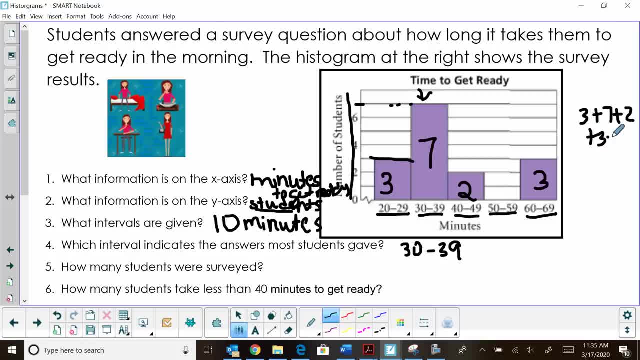 plus 2 is 12.. 12 plus 3 is 15. students took this survey. Then how many students take less than 40 minutes to get ready? Well, let's just kind of make ourselves a little line here: Everything to the left is less than 40 minutes, So we had 10 students that take less than. 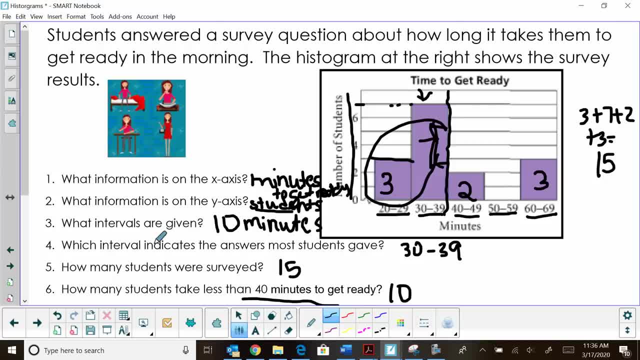 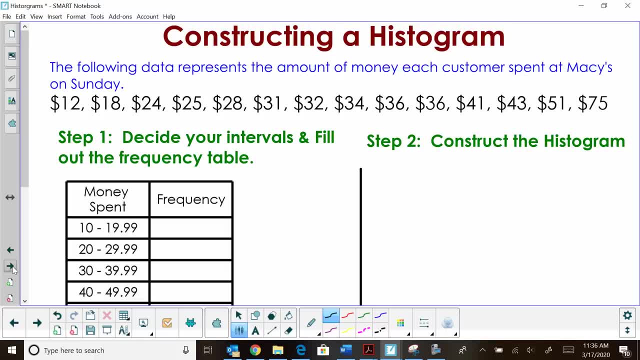 40 minutes to get ready. So that's how you interpret a graph or, in this case, a histogram. Now let's say we want to construct one. Okay, we're going to be given some data, We're going to have to take that data and we're going to have to make a frequency table out of it. 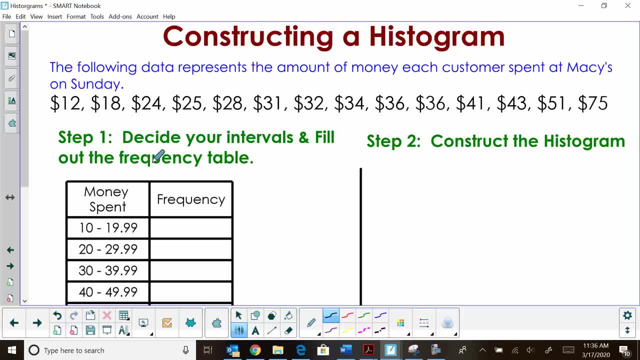 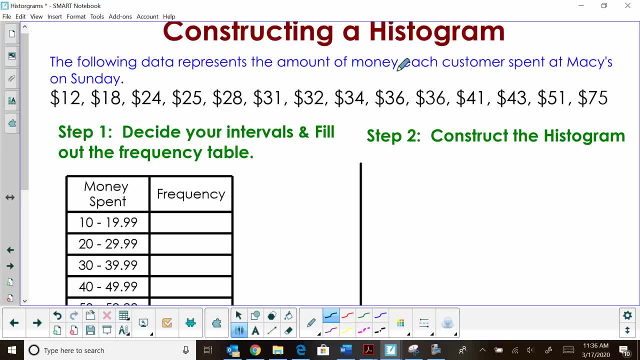 Then from that frequency table we're going to construct our histogram. So let's look at our data. The following data represents the amount of students that took less than 40 minutes to get each customer spent at Macy's on Sunday. We have 12,, $18,, 24,, 25,, 28.. So we kind of have to examine. 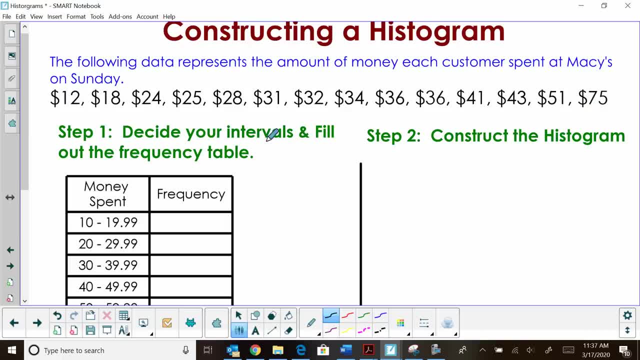 this data and see what kind of intervals we want to create. Well, it makes sense to group them in groups of 10.. So the money spent is going to be the left column of my frequency table. The right column is my frequency table, And that's what we're going to do. So we're going to do a lot of. dov. ¿no, This is a volta, and I just take the sugar out, So that's what I'm going to do. So let's look at the data students took last year and I'm going to take that so that the ratio is. 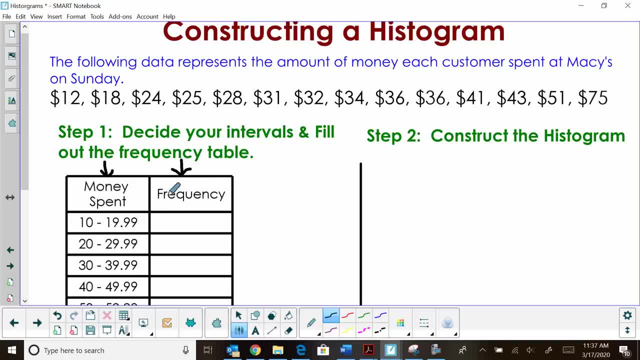 4 times where we took last year. We're going to take 12 using that integral of $20, and then I'm going to take this material and I'm going to be testing that. as I'm going to take, the is going to be my tally area where I can tally up the frequency of how much money was spent. 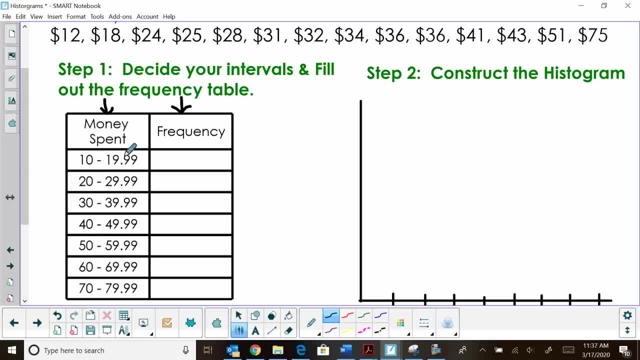 So I'm going to create $10 to $19.99. That's my first interval. Then I'm going to go $20 to $30, but I don't want to overlap, So I have to make that $29.99, and then $30 to $39.99, $40 to $49,. 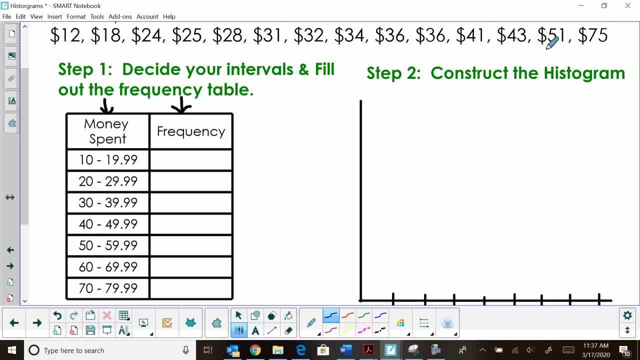 all the way up, all the way to $70 to $79.. Why do I have to go that far? Because my highest value is $75.. So now I'm going to take my data and I'm going to create a frequency table. So, $0 to $19.. 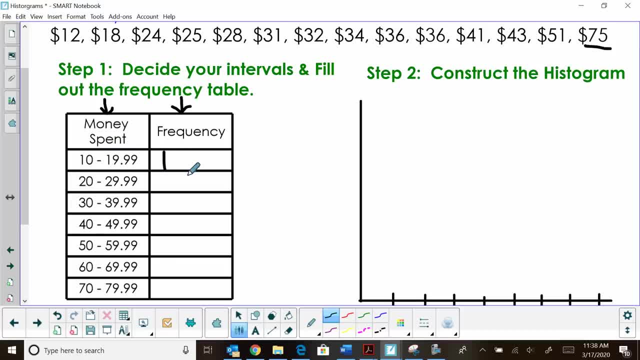 I'm going to look at the data. So I have one that's $12.. That's in that range, And then I have another one that's $18.. So I have two tally marks. Then $24 would go to $19.. 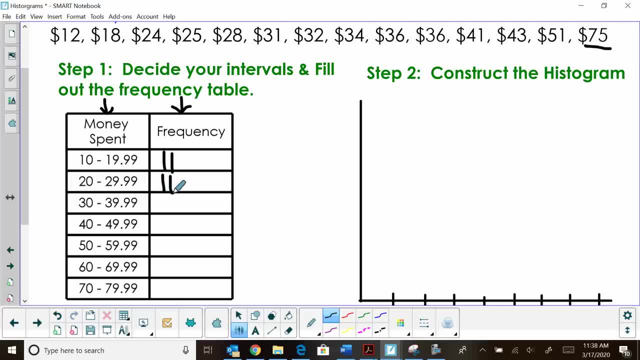 Go in this category. $25 goes in this category, $28 goes in this category. Now I'm up to my $30s. Okay, So I have a $31.. I have a $32.. I have a $34. And then two $36s, So that's five in that range. 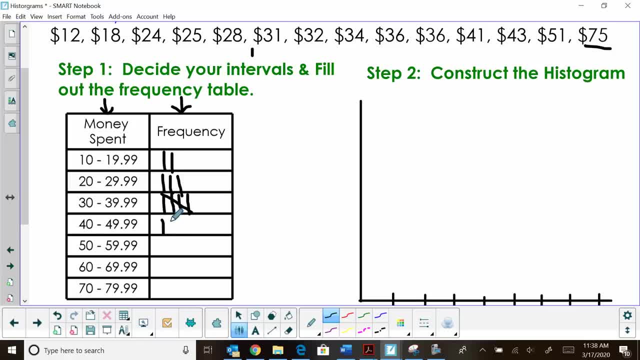 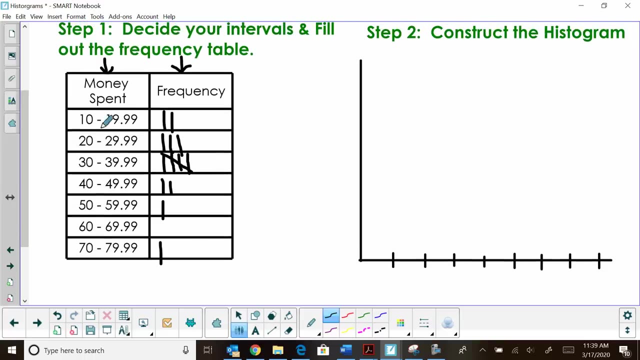 And then I have a $41 and a $43.. I have a $51.. I have any in the $60s And then I have a $75.. So here is my frequency table. Now I'm going to take my frequency table and I'm going to go over and create the histogram. So I have got to label. 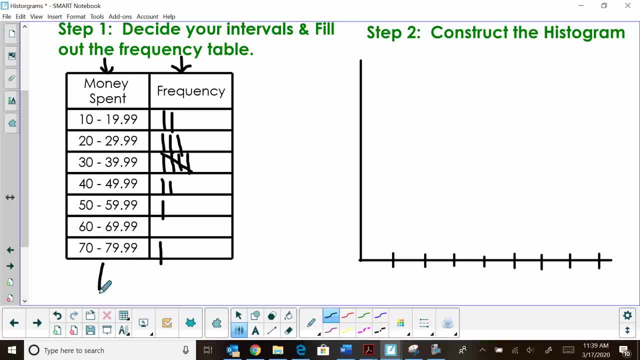 the x-axis in my money spent. My y-axis will be the frequency, which represents the number of customers. So I'm going to go over and create the histogram. So I have got to label the x-axis in my money spent. That's spent, that amount of money. So along the x-axis I've got to label that money spent. 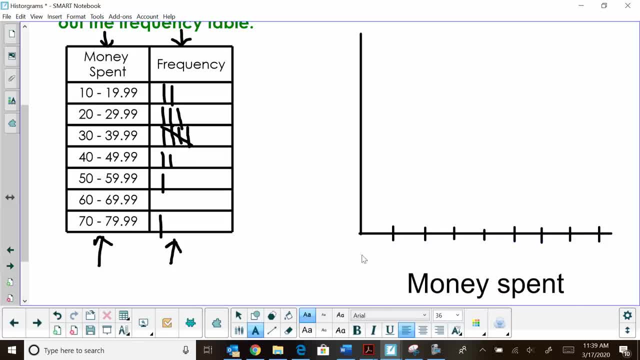 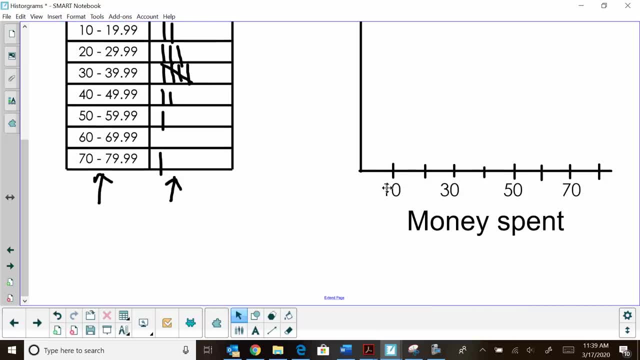 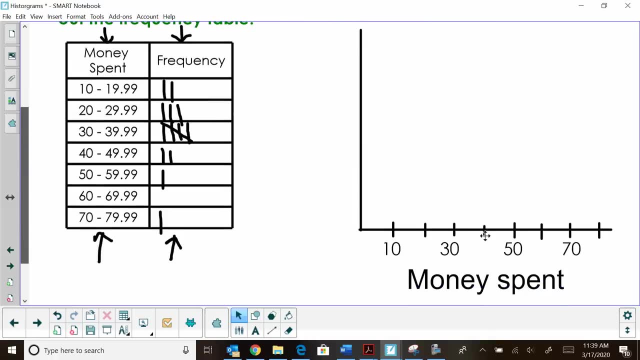 Now, not only do I need to label that interval with a title, I need to label each interval. So I'm going to label mine: 10,, 20,, 30,, 40,, 50,, 60,, 70, and 80, just like my table is labeled. Now it would be really tight for me to put. 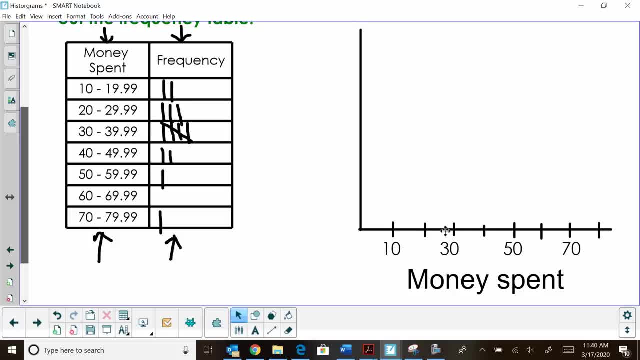 all 10, 20, 30, 40. So I'm just going to label 10 and 30 and 50 and 70. And everybody understands that halfway in between would be 20.. So now I need to label the y-axis. Now the y-axis is the. 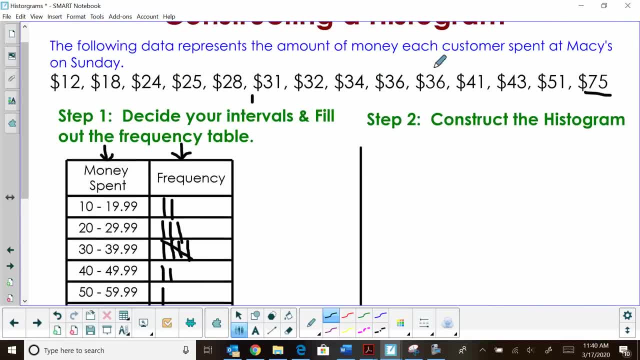 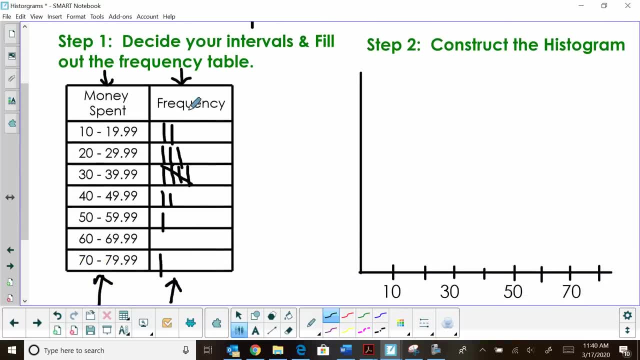 frequency that the customer spent money in those times. So I'm going to go over and create the intervals. So on this axis I am going to label from, my lowest value is 0 and my highest value is 5.. So I only have to label this y-axis 0 to 5.. So I'm going to make this 1,, 2,, 3,, 4, and all the way up to 5.. So I'll do 1,, 2,, 3,, 4, and all the way up to 5.. So I'll do 1,, 2,, 3,, 4, and all the way up to 5.. 1,, 2,, 3,, 5, and all the way up to 5.. So I'm going to label this: 1, 2,, 3,, 4, and all the way up to 5.. 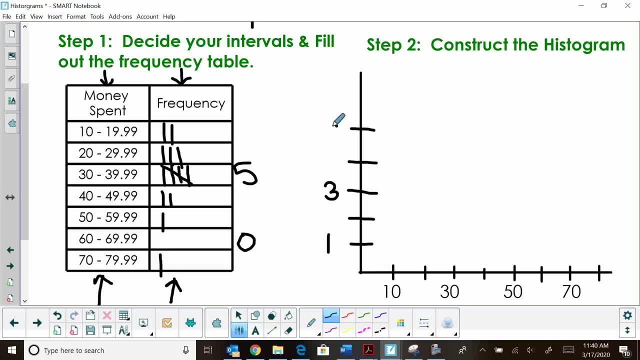 1,, 2,, 3,, 4, and all the way up to 5.. So this column does not, So this axis doesn't get too crowded. Now what does that represent? That represents the frequency of the money spent by customers. So I'm going to label that the frequency of the customers. 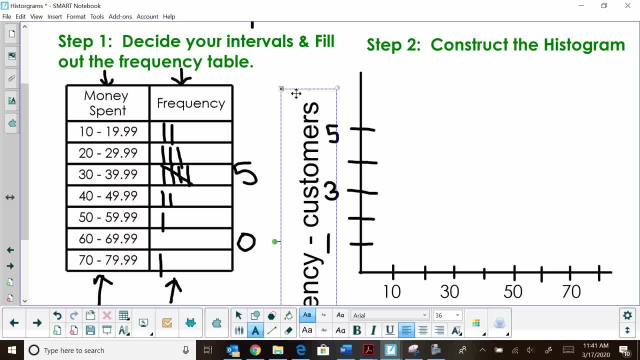 And let's true that, And I'm going to label this: 1,, 2,, 3,, 4, and all the way up to 5.. So I'm going to label this, turn that and move this over here to this column. I guess I could make that a. 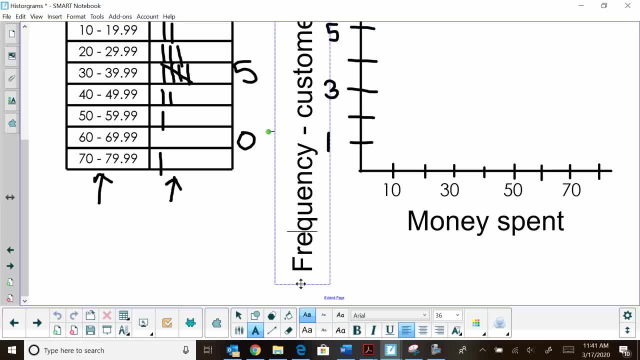 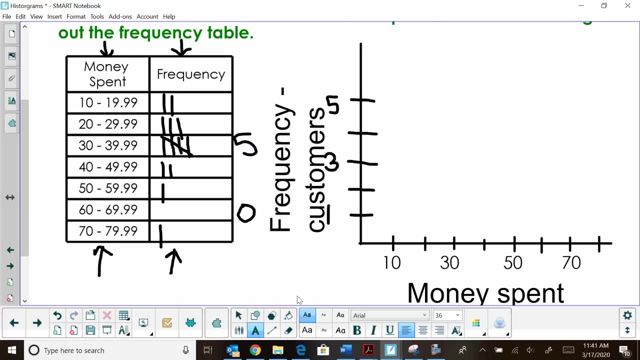 little bit smaller and you're gonna be writing these in, so they shouldn't be too bad. there we go. that fits a little bit better. so you want to make your table look really nice. now let's create our bars. so from 10 to 20 I'm gonna have. 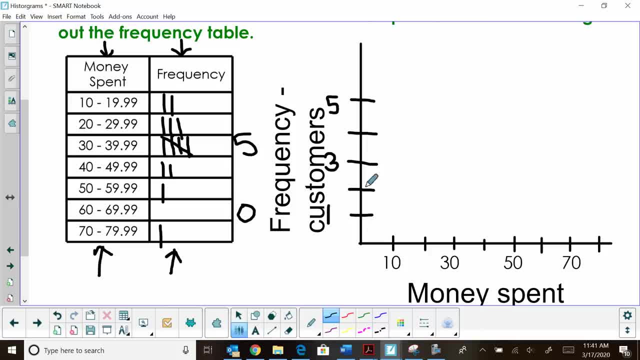 a bar that is has goes up to 2 because I have two customers that's spent between 10 and 20 dollars, and my next interval is 20 to 30 and I had three customers spend 20 to 30, so I'm gonna make my bar up to 3, then 30 to 39. that was my highest. 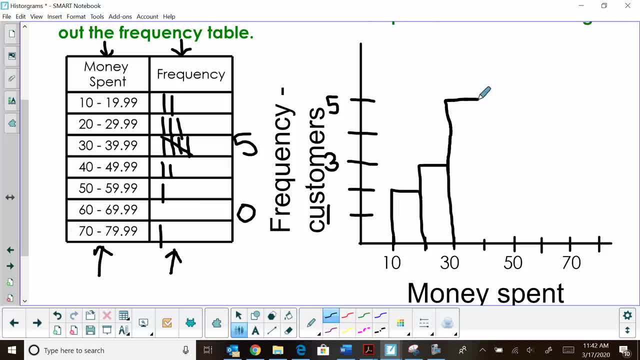 frequency. So I'm going to make that bar up to five, Okay, then 40 to 49.. I only have two in that interval, And then 50 to 59. I just have one. Then I didn't have anybody spend in the 60s, And then I had another one that spent 70 to 80. And there you go. So then you have your table.